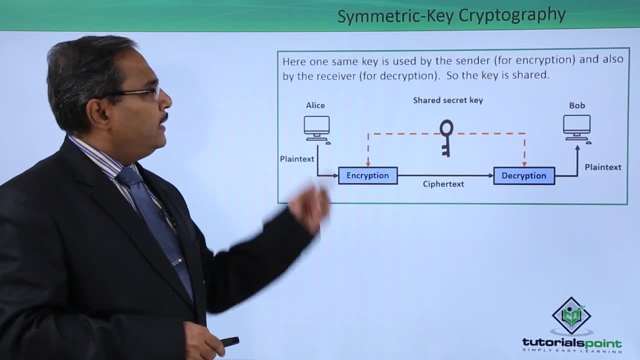 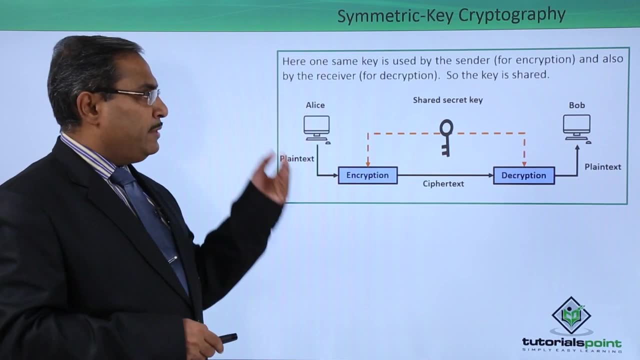 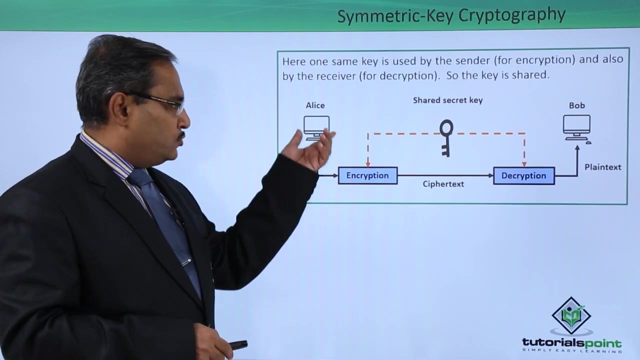 know that will be decrypted. So here one same key is used by the sender for encryption, and also the same key will be used by the receiver for the decryption process. So the key is shared. You can find this one. So here this is. let us suppose he is the sender and he is the receiver. So 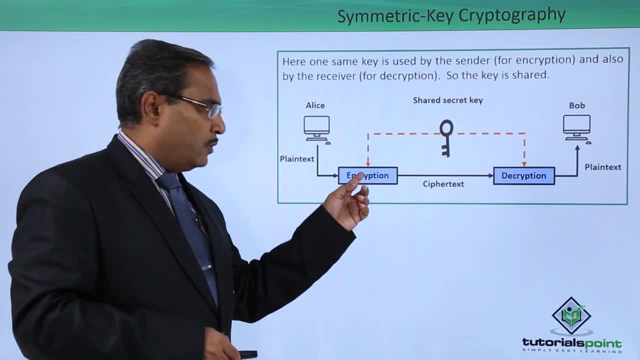 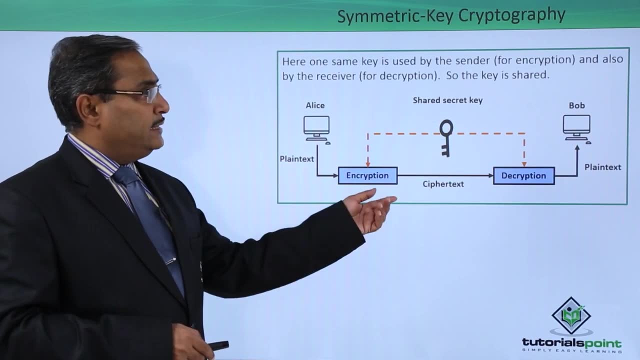 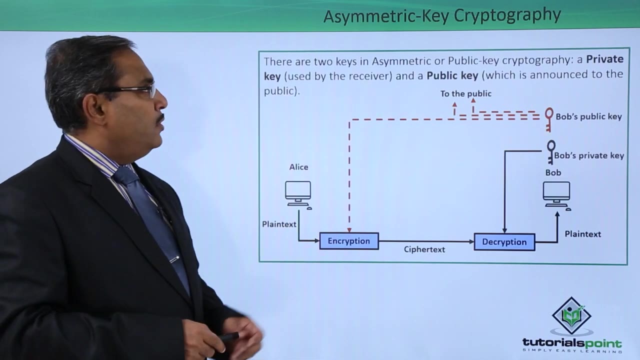 the same key, that is, the shared secret key, will be shared for both encryption and also for decryption, And here, through the media, ciphertext will be sent. And this is our symmetric key cryptography, the basic idea. In case of asymmetric key cryptography, there are two keys are there in asymmetric or public? 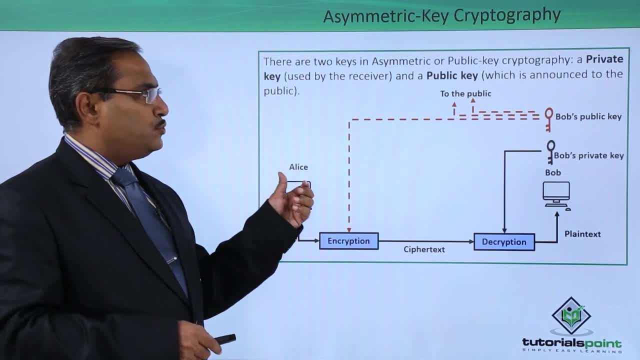 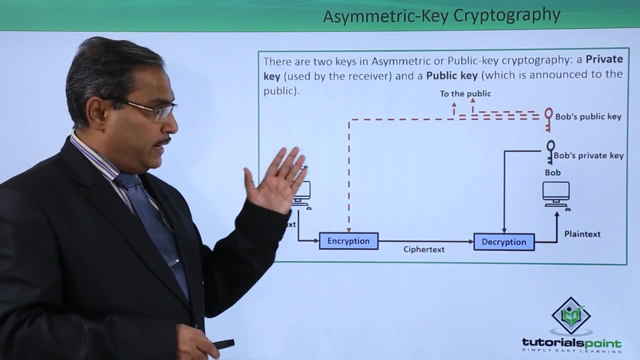 key cryptography. One key is the private key used by the receiver and another one is the public key which is announced to the public. So two keys are there you can find here. Here see, we are having this Bob's public key. So if I have a public key and I have a public, 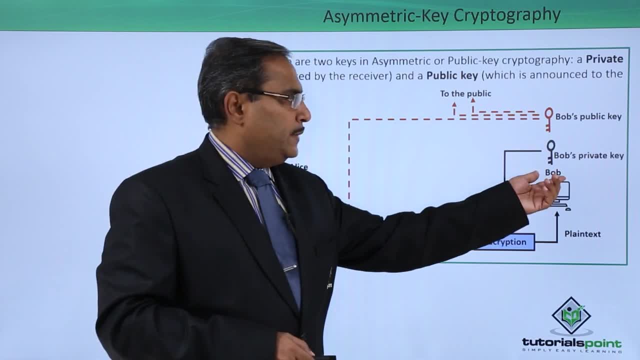 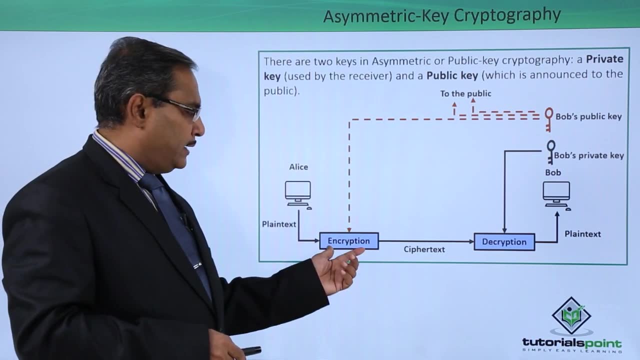 key which is announced to the public. So two keys are there you can find here Here. So this is the Bob's public key and this public key is available to all the public for this encryption. also, using the Bob's public key, it will be encrypted, The plain. 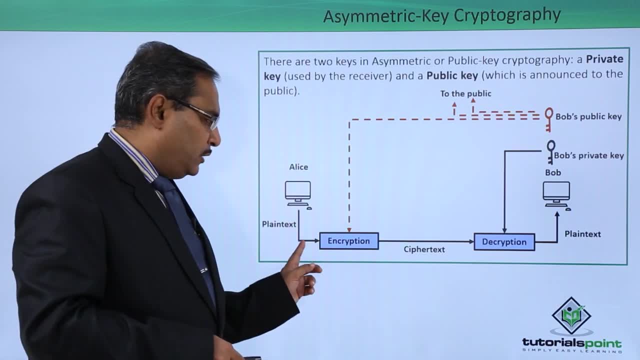 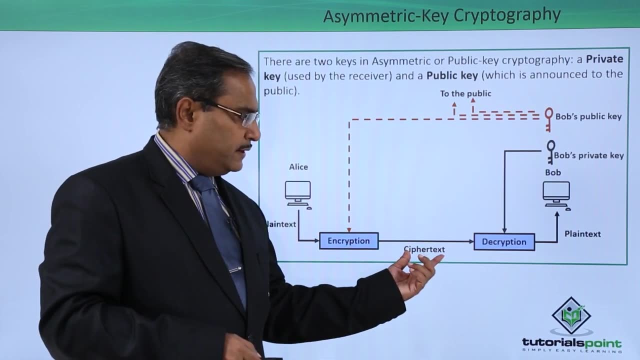 text will be there which is being sent by Alice, and this particular plain text is getting encrypted by the Bob's public key. Now it is getting transferred through the cipher text in the form and then at the decryption, Bob's private key will be used for the decryption. 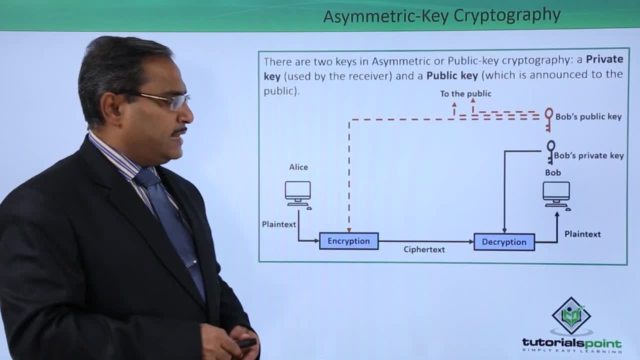 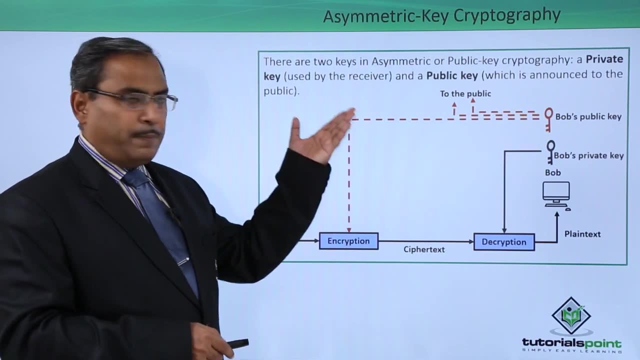 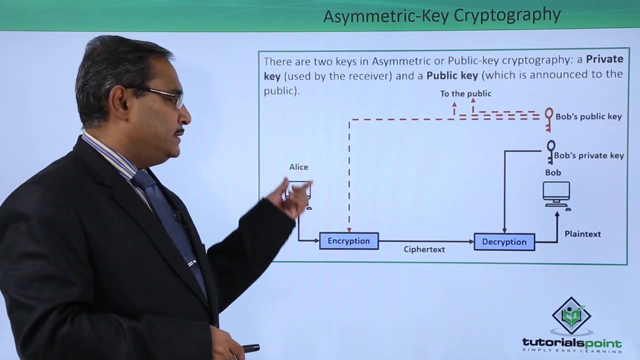 and then plain text will be originated. So this is known as asymmetric key cryptography. I think you are getting me. that means using the Bob's public key, which is known to the public, and that Bob's public key will be used for the encryption purpose. So, Alice, 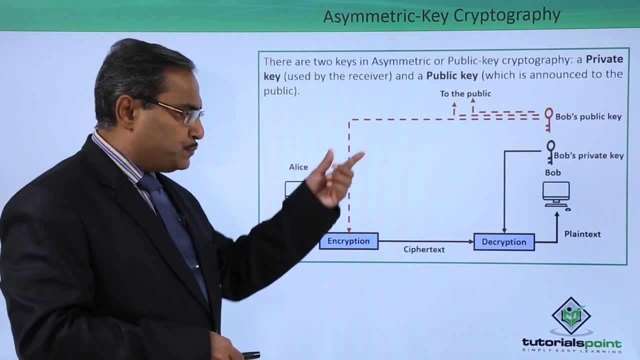 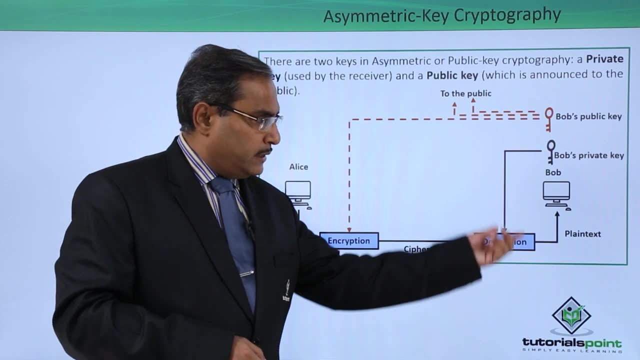 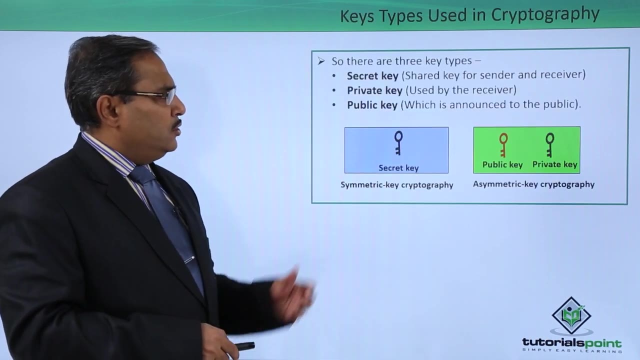 is a respective sender of the plain text using Bob's public key, it will be encrypted, So the cipher text will be originated, and then it will get decrypted by the decrypted by the Bob's public key. So the Bob's private key and the plain text will be re originated. So what is happening?